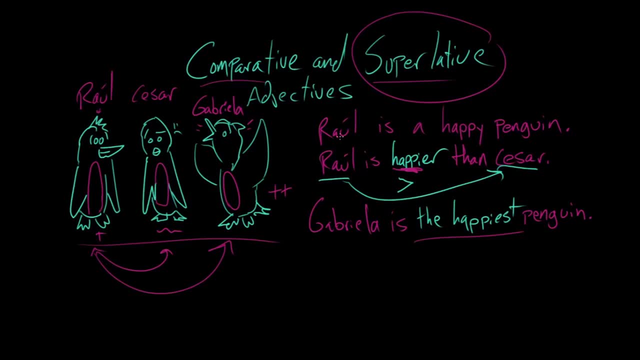 So it's not just a comparison, right, It's not. Raul is happier than Cesar. Gabriela is happier than all the other penguins. She is the happiest. She is the happiest, She's the most happy. So one way to think about this is that Raul's happiness. 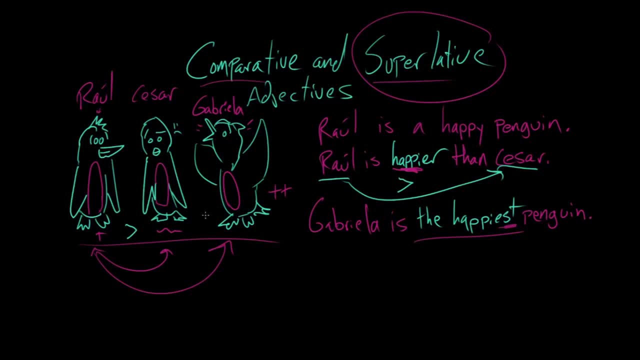 is slightly larger than Cesar's happiness, But Gabriela's happiness, this double plus, is unbeatably more than both of them, And I'm gonna use a made-up math symbol: Boop, boop, boop, Like super, greater than undisputed. 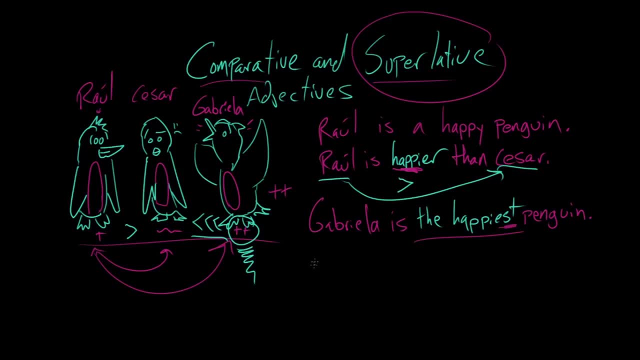 She is the happiest penguin because the comparative is the same thing as saying more. the comparative equals more and the superlative equals most. So this is slightly more. this is super much more, And something that's neat about English is you can use. 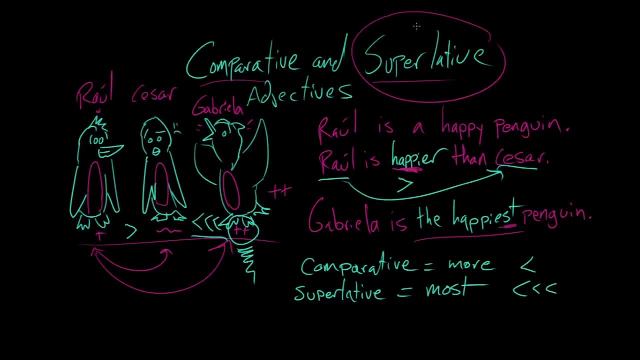 the comparative and the superlative for both positive relationships and also negative relationships. So we could say Raul is a happy penguin and we could say Raul is happier than Cesar. We can also say Cesar is less happy than Raul. 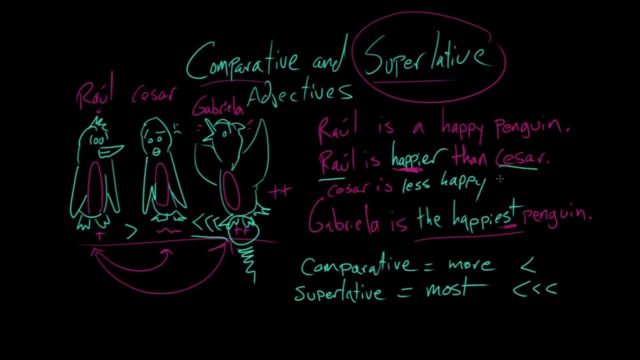 We can also say: Cesar is less happy than Raul. We can also say: Cesar is less happy than Raul. So this is comparative, but it's going the other way, Cesar is less happy than Raul. so then we'd use: 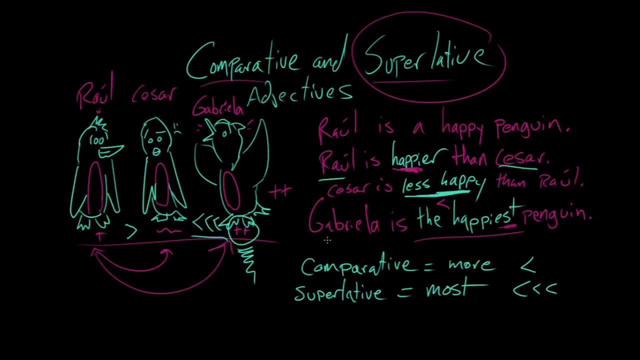 the less than symbol. Gabriela is the happiest penguin, and so, for this group of three, Cesar is the least happy. Cesar is the least happy. So you can use the comparative and the superlative forms of adjectives to compare relationships where one thing is: 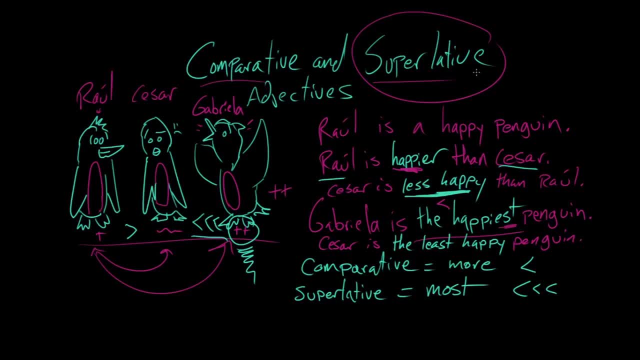 more or most than another, or others, or relationships where one thing is less or least than others. That's how the comparative and superlative work. but if you stick around for the next video, I'm going to talk about how to figure out, how to form the comparative.